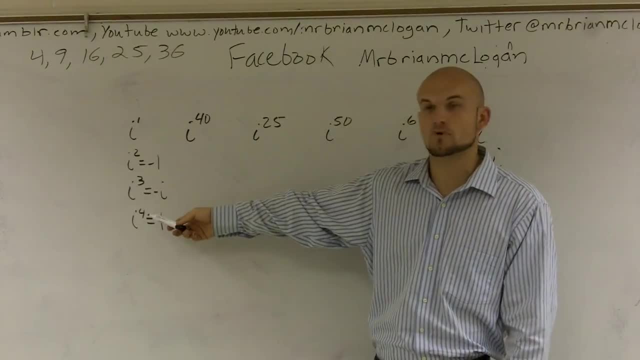 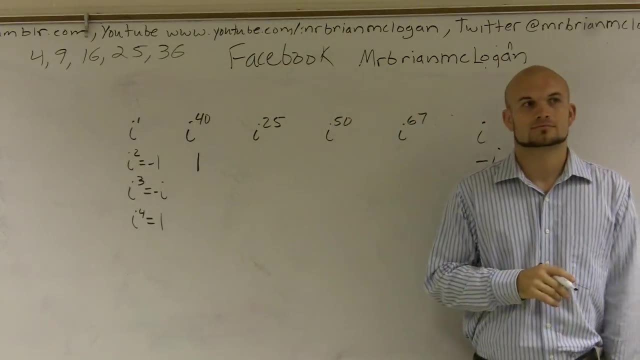 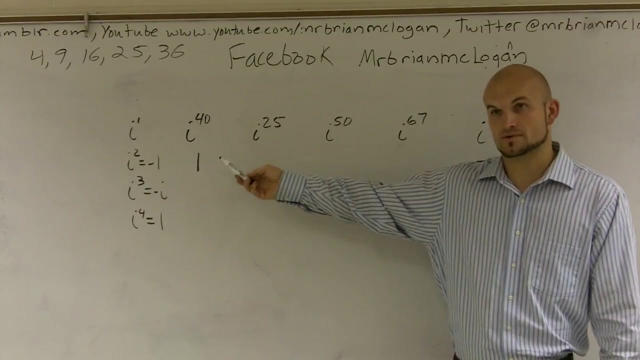 No, So therefore, a remainder is going to be 0, or what we call 4.. So, therefore, this can be rewritten as 1.. Okay, i to the 40 is exactly similar to 1, or i to the fourth: It's the same thing. 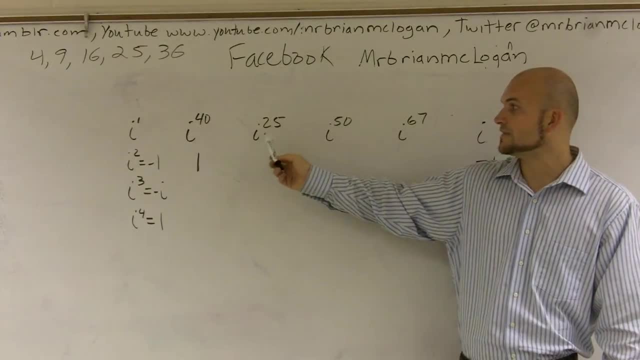 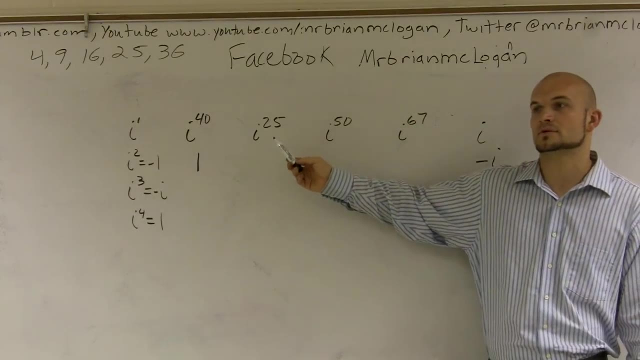 as i to the fourth, which would equal i to the first power. If I looked at i to the 25th, how many times does 4, four options? how many times does that go into 25?? Six times right. 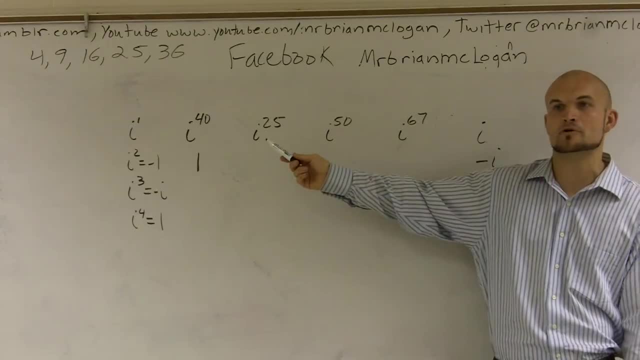 But it just keeps on repeating that six times. Then, after that six times, what is my remainder? 1. 1. So, therefore, this is going to be: we can put it into 4.. So what we're going to do is: 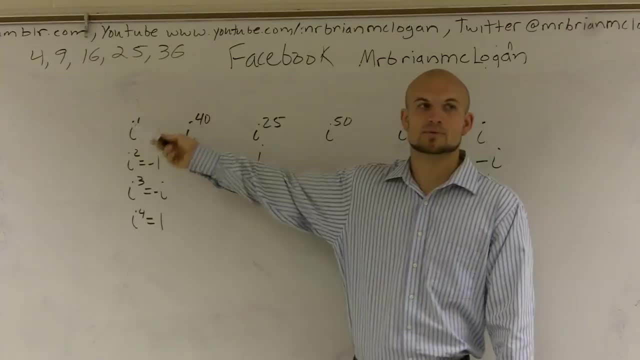 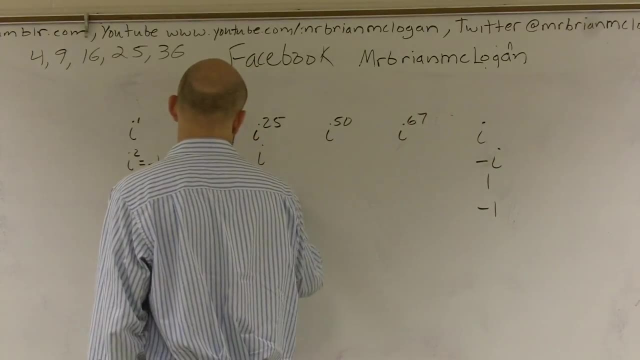 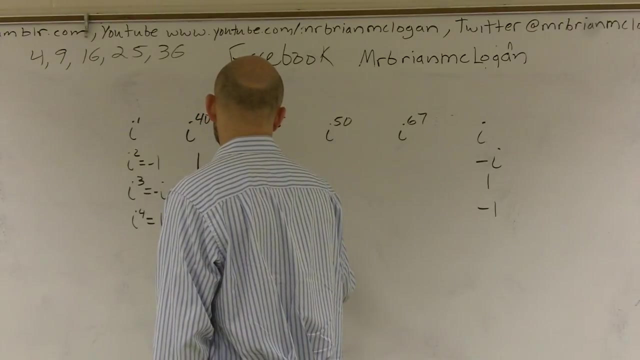 we can represent this one as i. Since I have a remainder of 1, I represent it as i. Does that make sense? Let me put it to you this way: Let's add in i to the fifth right. You can write i to the fifth as i to the fourth times, i to the first power right. Well, i. 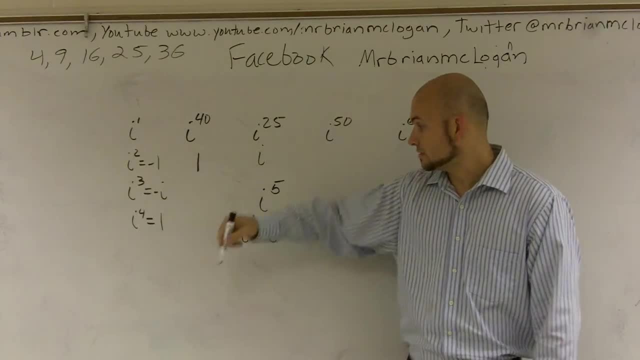 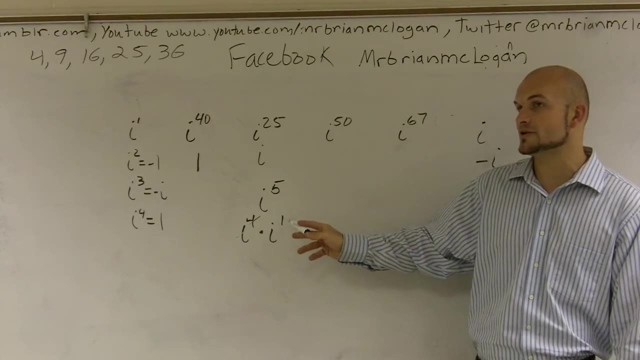 to the fourth is just 1, right, And then you're just left, with i to the first power. So you just take what the remainder is, Bless you. You're just going to take what the remainder is and that's going to tell. 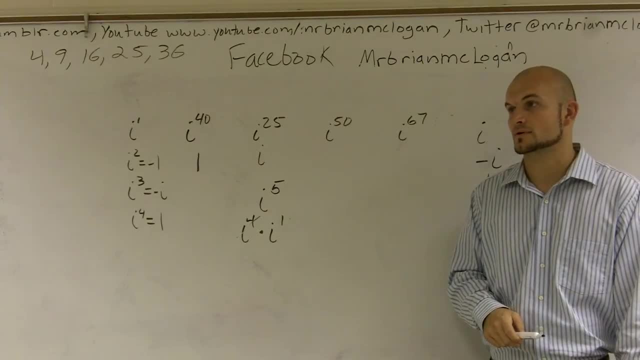 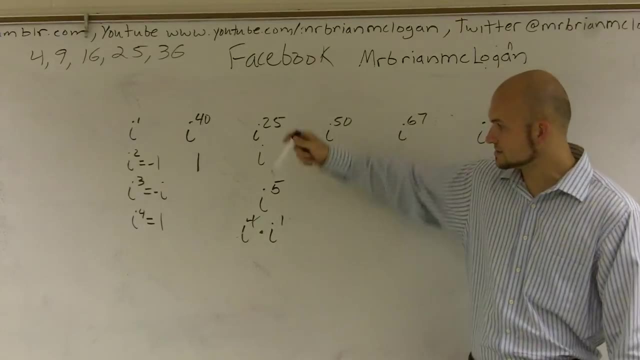 you what you can rewrite that power as: Yes, So after you get from i4 to i5, does the cycle just basically repeat itself? Yeah, I mean, this is just like cancer. Let's look at i to the ninth. Again, you can rewrite: 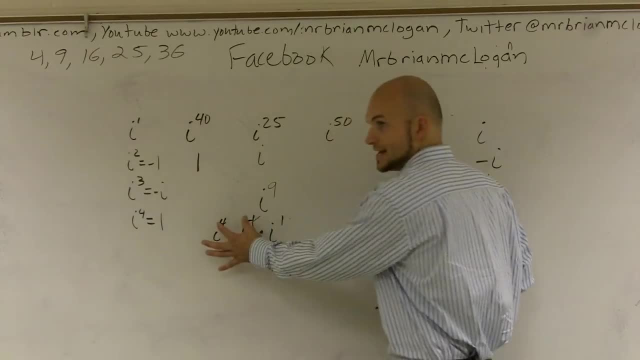 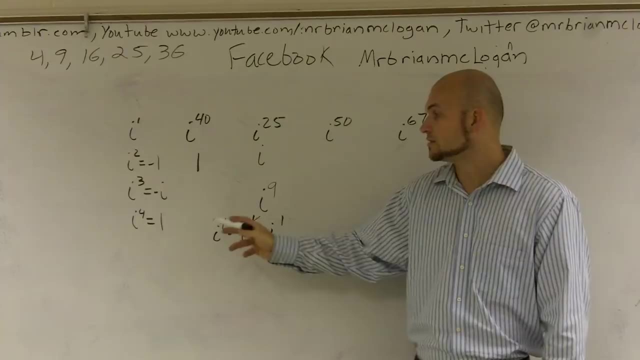 that, as i to the fourth times, i to the fourth. Remember you add exponents right: 4 plus 4 is 8, plus 1 is 9.. Well, what do these both equal? i to the fourth: equals what: 1.. So 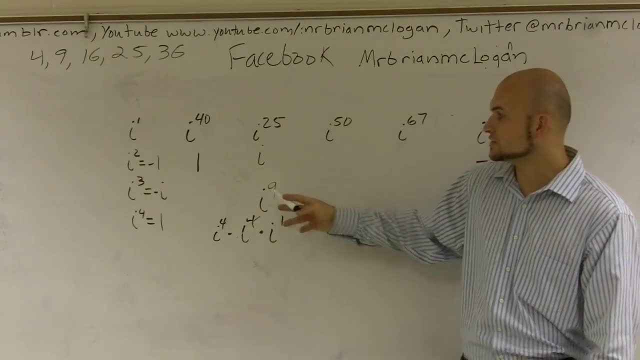 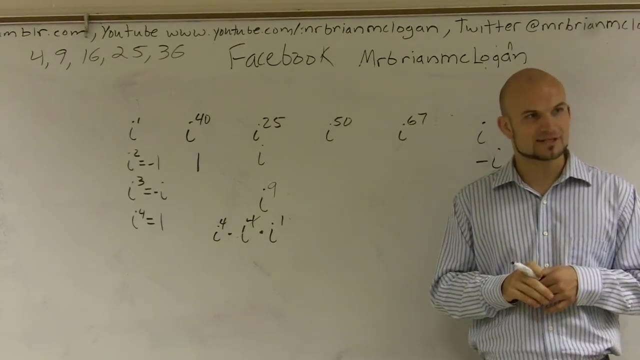 it would be 1.. 1 times 1 times i. So that's why I can rewrite i to the ninth as just i. So basically, you divide it by 4, and whatever the remainder is is what To make it in simplistic terms. yes, 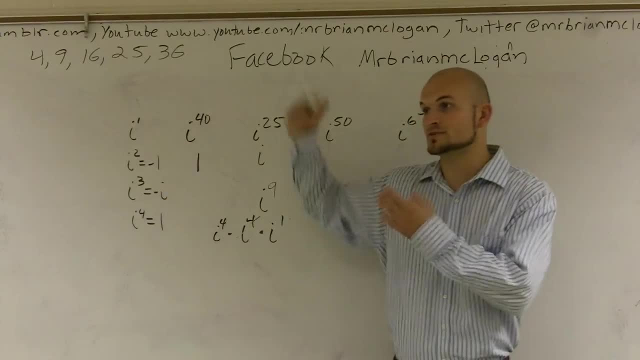 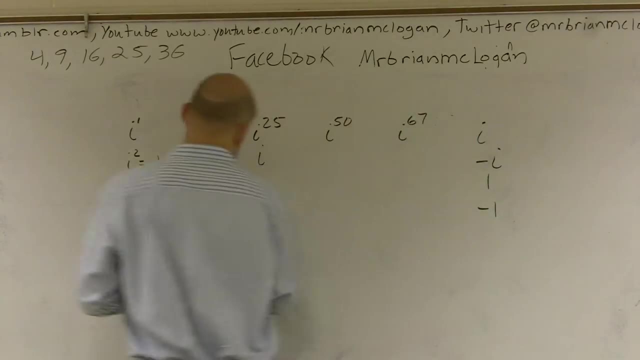 You always divide by 4?? Yes, because there's only 4.. Because once you get up to 4, it resets right, Or you could spend your time counting. I would just want to do that. That's a lot easier. 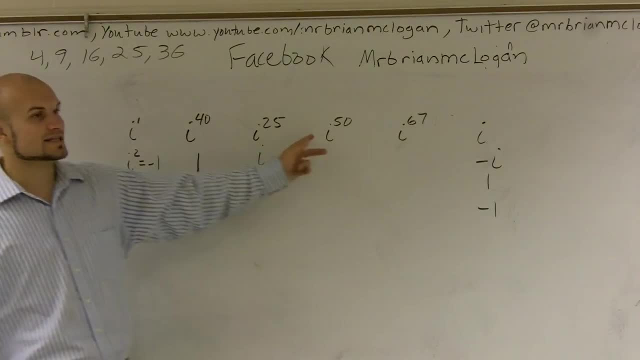 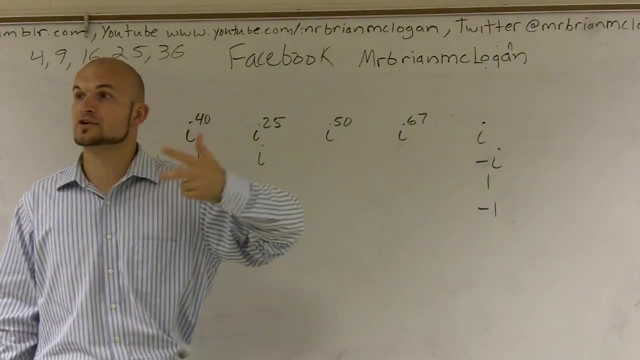 It's a lot easier to divide by 4 and find the remainder. So i to the fifth. we look at this and we say: how many times does 4 go into there? Well, 12.. 12 is going to give us 48, so my remainder would be 2.. 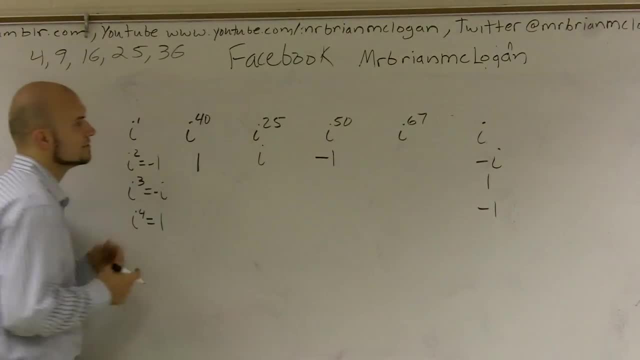 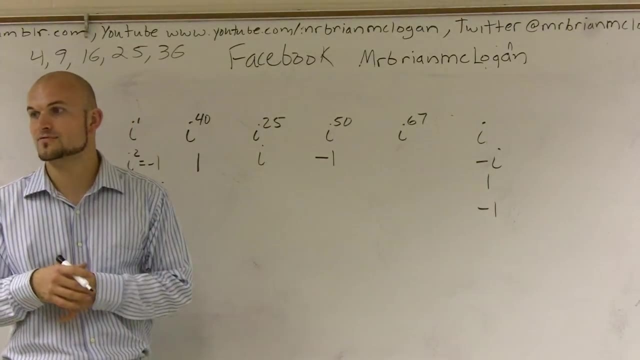 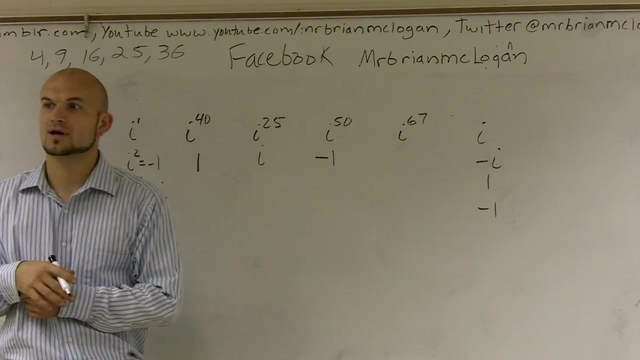 So my remainder of 2, this can re-re-re-re-reset as negative 1.. 67, i goes into there. well, 4 goes into 40 10 times. and then what? 24 would be the next time. so then, 10 plus 16?. 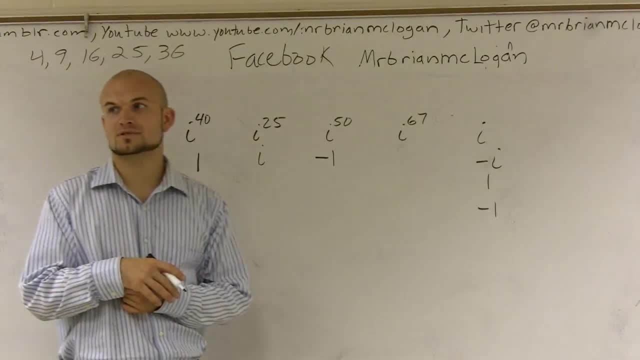 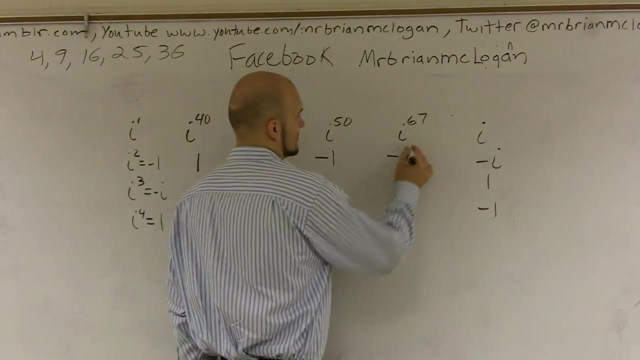 16 plus 7, 5? 16.. So what's the remainder of 4 times 16?- I don't know- 64, so it would be a remainder of 3, so it would be negative. i I still don't get that. 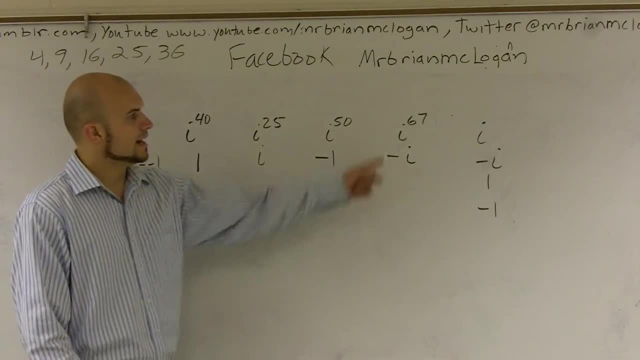 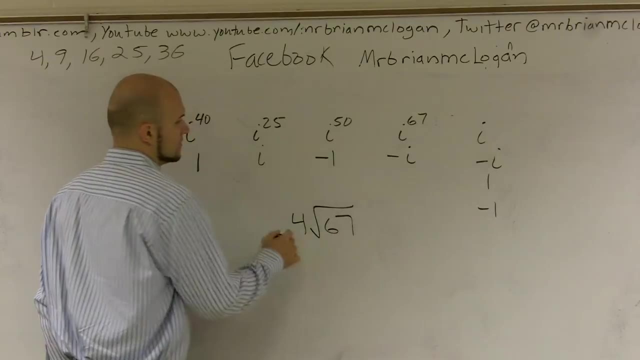 I can't tell you. Yeah, you're confusing me. How many times does 4 go into 67?? Let me see Watch. Wait, no, that's just so confusing, Mr McClugin, don't do that. 4 goes into 6. how many times? 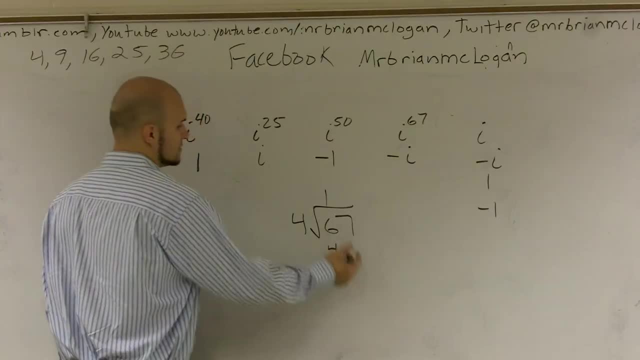 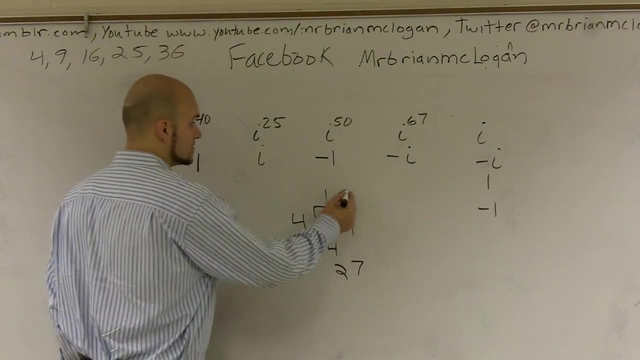 16.. 1, 1 times 4 is 4, drop it down 2 goes into 27. how many times 4 goes into 27.. 4 goes into 27.. 6 times 4 is 24,. my remainder is 3, right. 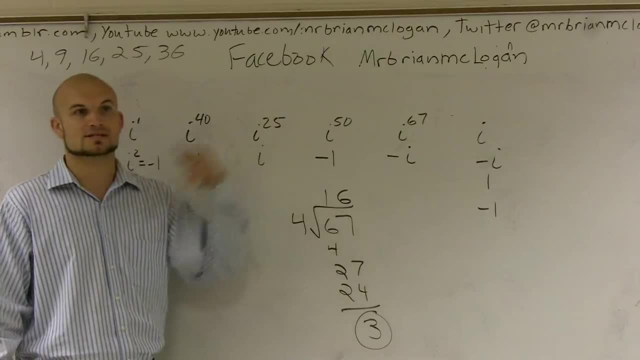 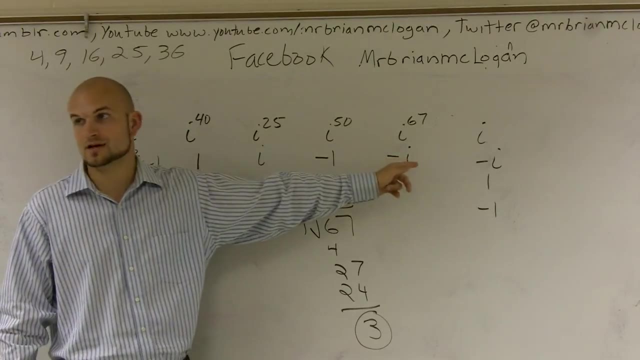 It goes in there 16 times. that means it repeats over 16 times. but then I have a remainder of 3.. We take whatever our remainder is and that's our exponent, so it's i equals negative 1.. Then it's i to the 4th, because it's repeated. 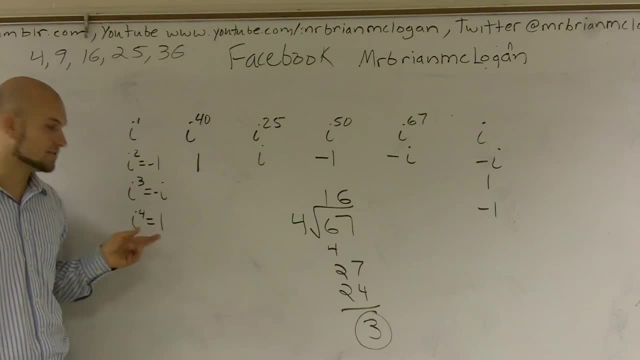 It's just 1.. It's just 1.. If you don't have a remainder, then it's i to the 4th power. So can't we just count? You can. You can go ahead If you want to count all the way to 67,. we want to guess. 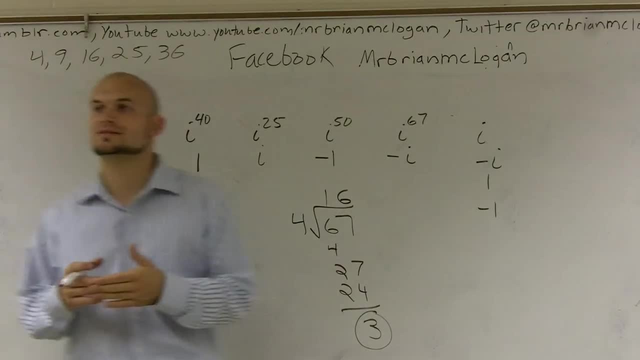 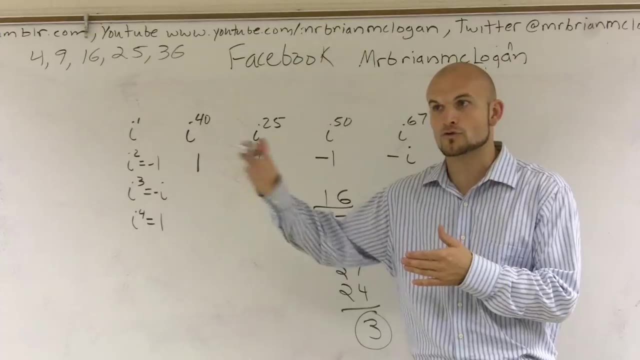 Right, But all you're doing is counting. It's the same thing, Jessica. it's the same thing. like this, It's so much faster. But if you're counting, multiplication is just doing addition over and over, right, Right.